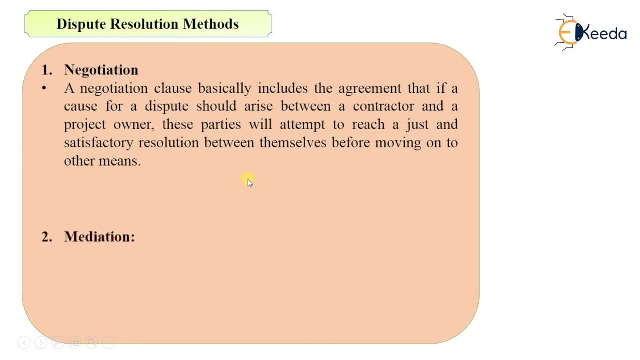 resolve the issues by themselves. That is the negotiation. Then we have mediation. Mediation means a clause that suggests inclusion of a neutral third party in the dispute situation to help mediate the process of resolving the dispute. See in the first case of negotiation. 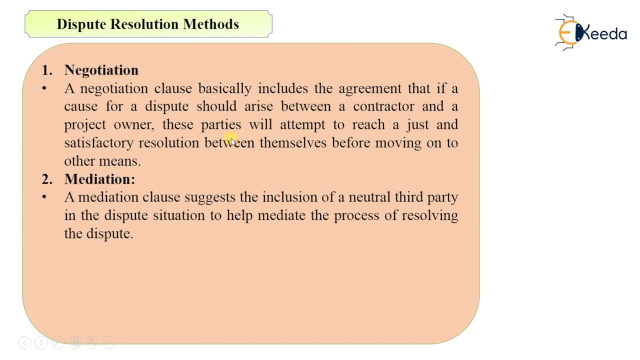 there will not be any intrusion of the person. The matter will be solved by the parties themselves, But in mediation there will be a third party. there will be a third person that he will mediate between the process and he will try to resolve the dispute. And see, mediation is not legally. 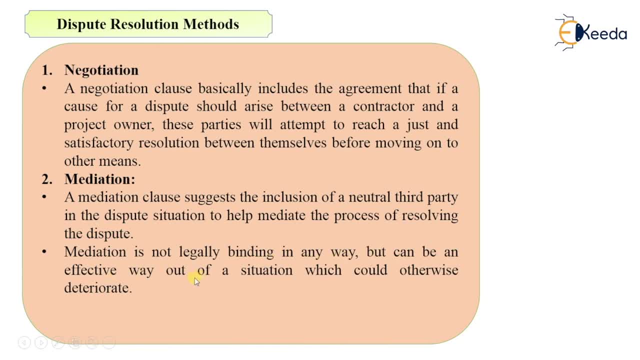 binding in any way, but can be an effective way out of a situation which could otherwise deteriorate. So mediation is not considered to be a legally binding in any way, but it is obviously the effective way to solve an issue. If you are using a third party person, then you can solve that. 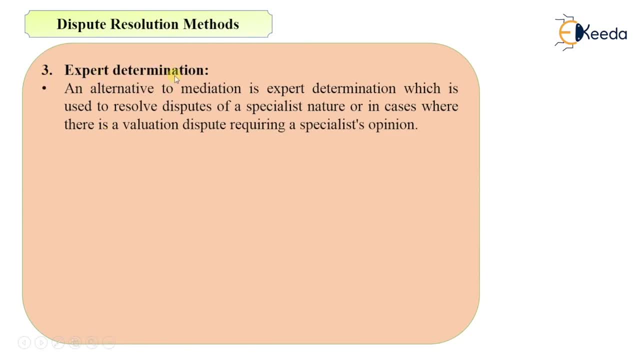 particular dispute. And then we have expert determination. This is the third method of dispute resolution. Now, what it includes see, as the name says, expert determination. the alternative to mediation is expert determination, which is used to resolve disputes of specialist nature or in cases where there is a valuation dispute requiring a specialist's opinion. 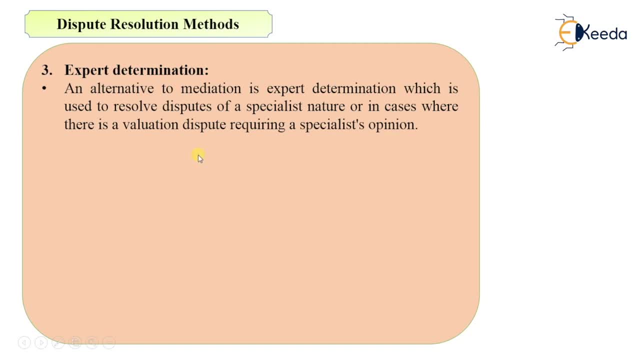 See if mediation is not enough, a mediation person who is not expert to solve that particular issue, if any technical expertise is required, any expert determination is required, then in that case there is third method. we have Expert determination, in which that particular dispute or issue will be solved by a specialist. 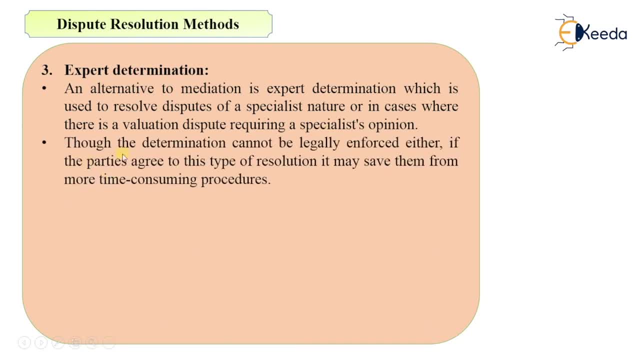 if particular special work is there, Then, though, the determination cannot be legally enforced either. if the parties agrees to this type of resolution, it may save them from the more time consuming procedure. See, it is also not considered or cannot be legally enforced, but if both the parties are ready to take the expert determination, they can resolve the dispute. So if the parties agree to this type of resolution, it may save them from the more time consuming procedure. See, it is also not considered or cannot be legally enforced. but if both the parties are ready to take the expert, 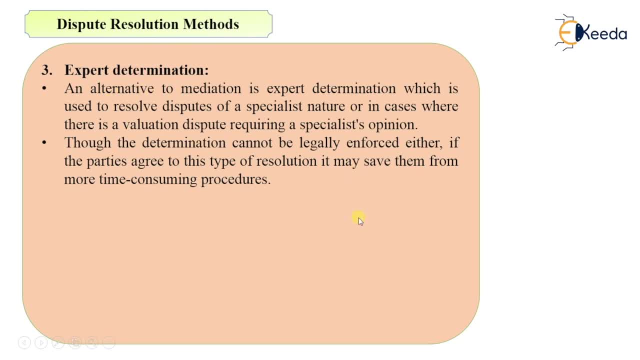 determination and solve the issues by using this method, then it is well and good, because their time will be saved. Then we have adjudication. Now what is adjudication, See? it is a method that includes a neutral third party. See, in expert determination, we also including 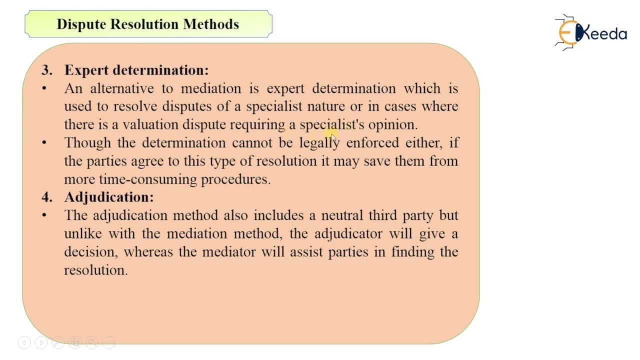 we are also including a third party, but it will be a. he will be a specialist, he will be an expert. Then what is adjudication? See, it includes a third party, but, unlike with the mediation method, the adjudicator will give a decision, whereas mediator will assist the parties in finding. 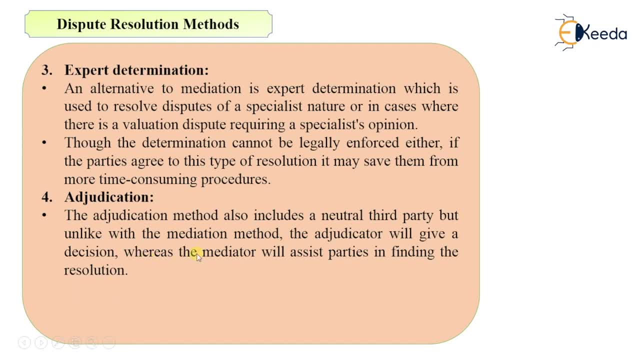 the resolution. That is very important. We have seen what is mediation. It is in mediation, mediator will assist- just assist- the parties. He will help the parties to find a resolution. Now. mediator is also a common solution, but in adjudication, an adjudicator will give a final. 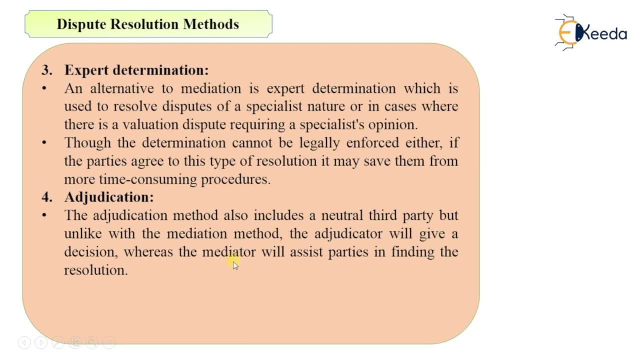 decision. That is the difference In mediator. he is giving the resolution, he is, he is finding the solution and he is capable of giving the decision. This adjudicator. that is the difference, and adjudication clauses typically also include the possibility of applying. 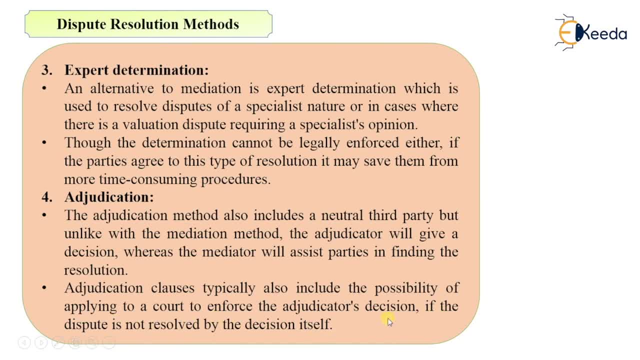 to a court to enforce the adjudicator's decision. if the dispute is not resolved by the dispute is not resolved by the dispute. That is the difference decision itself. if, for example, adjudicator made some decision but both the parties are not expect accepting that decision, so what will happen? this decision can be taken in the court of law. it can. 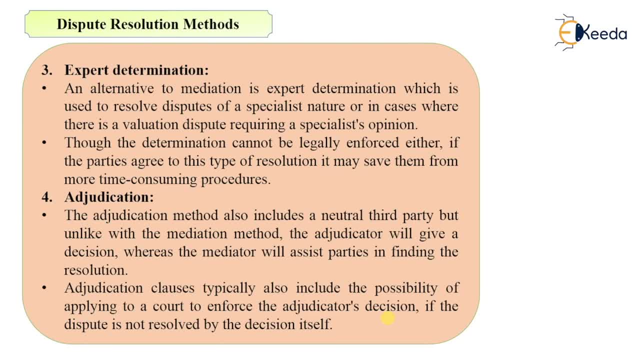 be enforced in the court of law and possibility can be find out whether it can be accepted or not by the court. so if it is not getting solved between these parties by the adjudicator, then it can be enforced in the court of law. this is the fourth method of dispute resolution method. 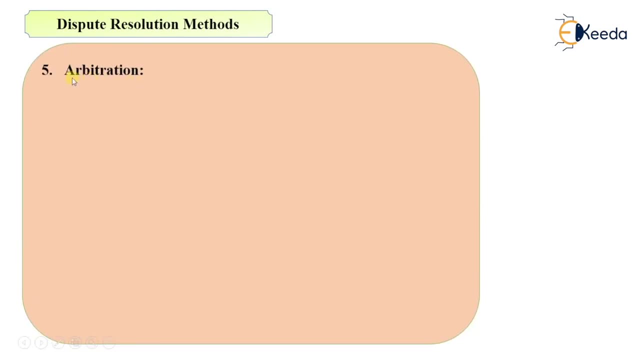 then we have arbitration. see, it is one of the most famous methods. you can say: if parties decide to go for arbitration, they will again have a neutral third party enter the situation to help resolve it. see, in this method also, there will be a third party to solve the issue or resolve the issue or resolve the dispute in 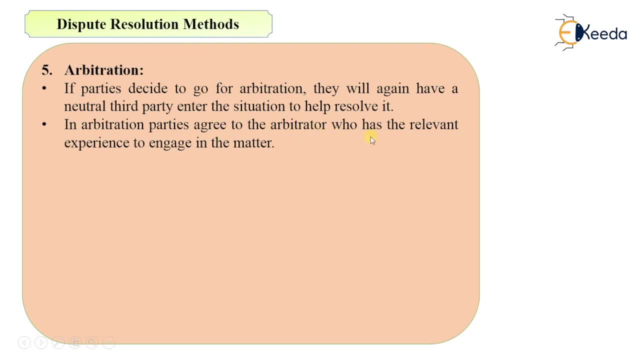 arbitration, parties agrees to the arbitrator who has relevant experience to engage in the matter. he will be an experienced person of that relevant field and parties will agree to a final decision which is made by the arbitrator. arbitrator is nothing but that person who will help them in. 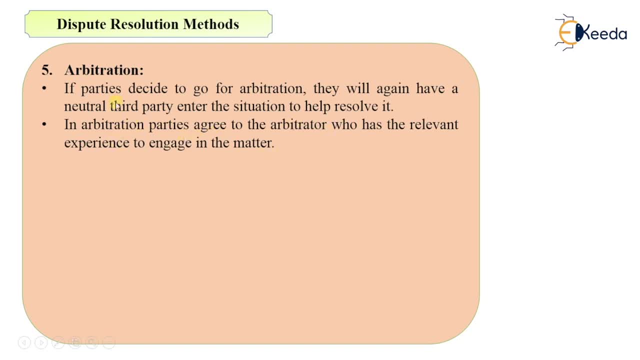 finding of common or final solution. arbitration. now, who is arbitrator? he will listen to the board parties and he will make one, made one conclusion and that has to be accepted by the parties. the arbitrator, what he will do? he will consider the documents, he will listen to the facts of the owner and the 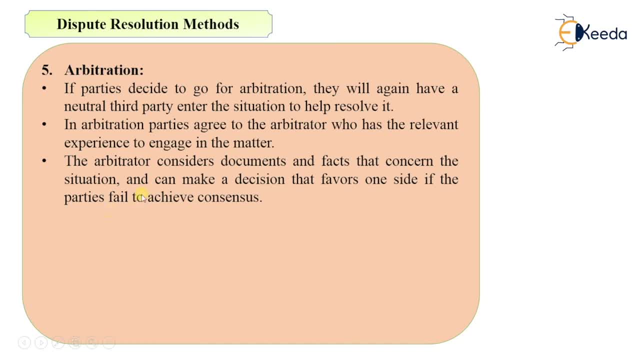 contractor two parties. he will concern the situation and then finally he can make a decision that favors one side. if the parties fail to achieve the consensus, see, if parties are not capable of taking a final decision, then arbitrator will check the documents. he will listen to the facts by both. 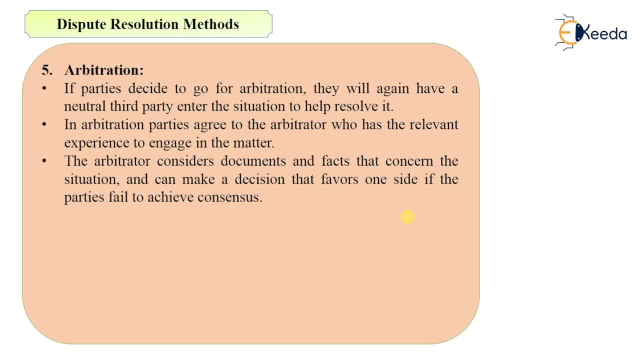 the parties, he will analyze the situation and finally he will make a decision only in favor of one side in the one party. after reading all the documents, after going through the meetings with every host for five minutes, then the gr chemotherapy has finally going to give thespace B most important. 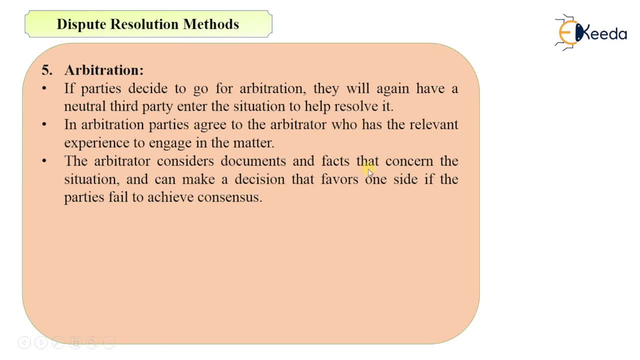 after reading all the documents, after going through this, documents faxed and all this, you will make a decision and arbitration can be legally binding depending upon the jurisdiction. in which jurisdiction are you. depending upon that, even arbitration can be a legal binding. the cost of arbitration can be significantly higher than that of other methods. 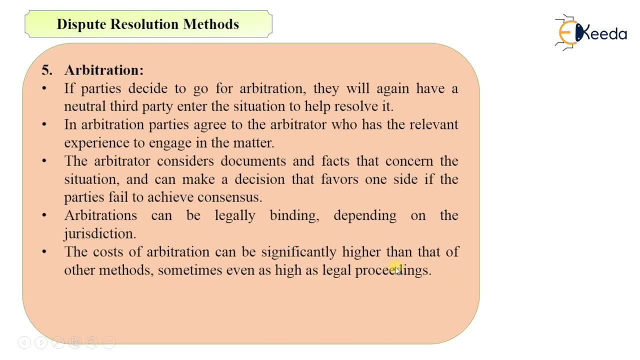 sometimes even as high as legal proceedings. see it why generally people will not go directly with the arbitration? because it will be costlier. because that methods which we have seen in the previous slides, then this method, that arbitration method, is costing somewhat higher side, so that's why it will. it can even cost them as high as legal 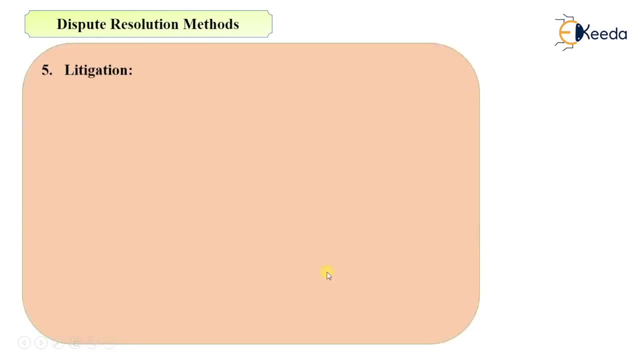 proceedings. then we have six one litigation. now, what is litigation? they see? finally, it is usually also included in the dispute clause in case of parties do not find any other way to resolve the issues that have come up. so litigation involves a trial and is legally binding, an enforceable, though it can also be appealed. 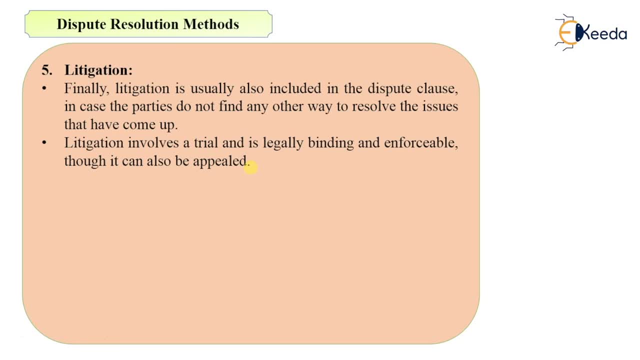 see. Finally, rev No Cen 3250.. accepting any, any of the methods above, still the issue is not solved, then in that case litigation will be followed. it is nothing but trial and it is a legally binding enforceable by the law and it can. but it can be appealed and see, litigation can be by far the most thorough. 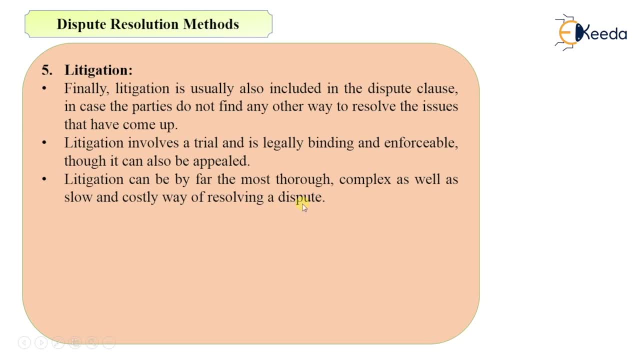 complex as well as slow, costly way of resolving a dispute. it is nothing but solving a case. it is similar to like solving a case. it will take trials and trials. it will take time, it will be a slow process, it will also cost to the both parties for solving a particular dispute and finally they will 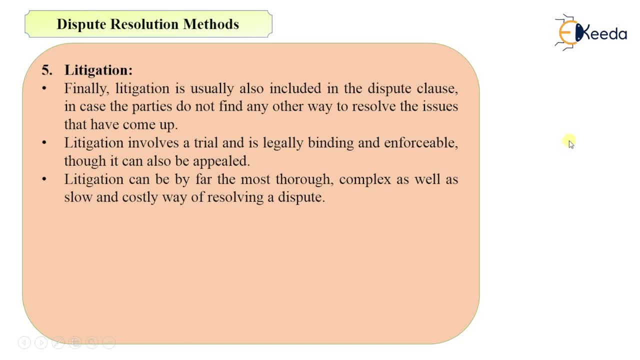 come to the decision and that is legally binding. it is enforceable by the law. that is what litigation is. so this is the fifth method of dispute resolution method. so this is why parties will typically attempt a number of other resolution methods before opting for litigation. why? why we will. they will have the 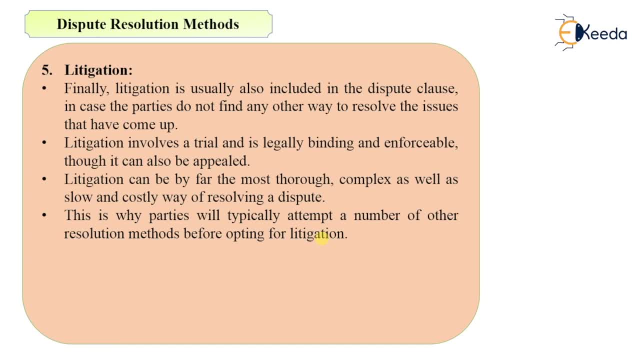 finally, the litigation option. final option will be litigation. why so? because it is time consuming, it is costlier, so that's why it is also very complex process of litigation. therefore, they will consider it as a final option in case of dispute, dispute resolution. so this was the